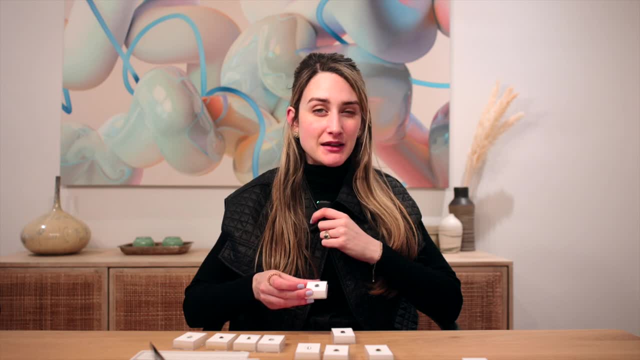 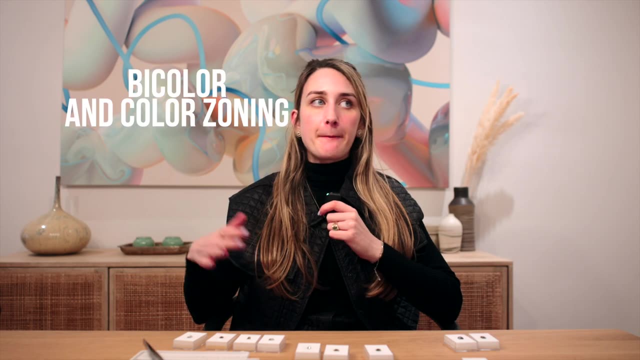 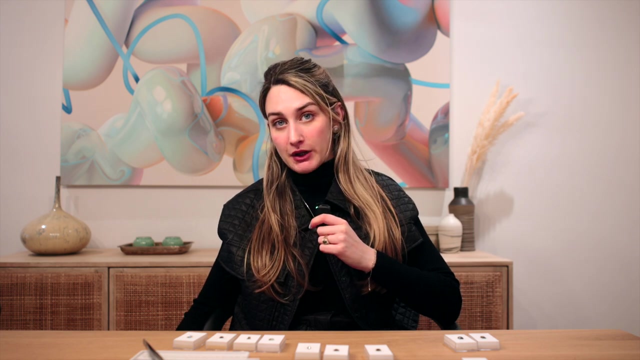 a little bit more blue. So there's still. I would still consider them in the teal family, but it gives a very different aesthetic completely. Now let's look into kind of like bi-colored and colored zoning. So a lot of the teal sapphires come from Montana and they come from Australia Like by a. 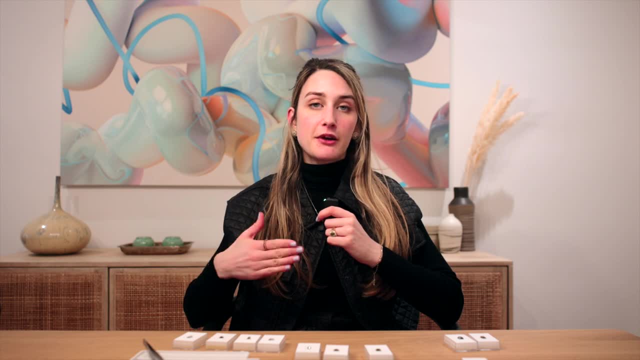 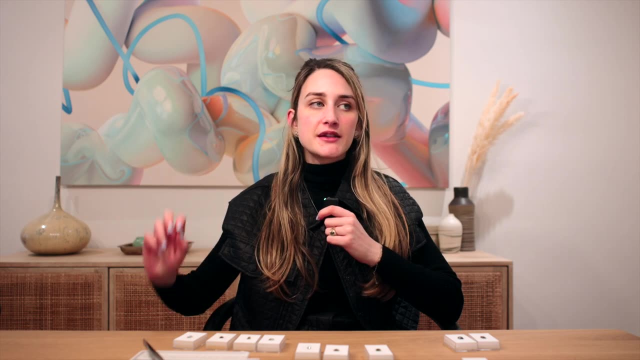 default. anytime I'm looking for teal, they always tend to be coming from these places. Of course there are others like Madagascar. you know it's not exclusively to that, but they kind of like triumph in those colors, And a lot of the times I find that they will have bi-colored. 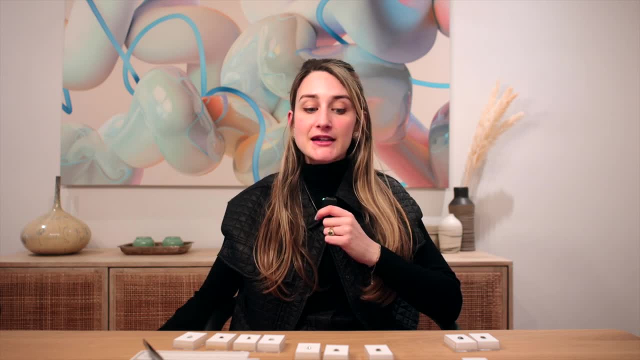 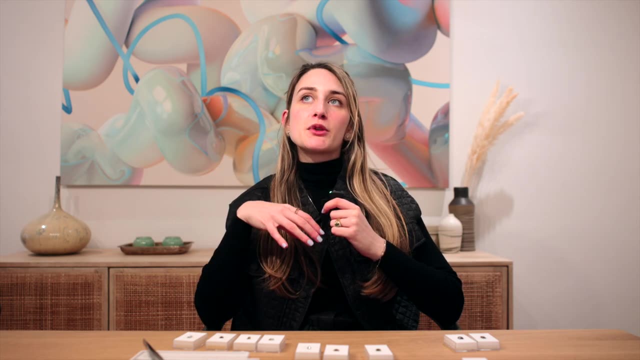 tri-colored or color zoning within the stones, And this is really beautiful, In my opinion. I would definitely look for a stone that has these kinds of tri-colored properties, because it just gives so much more nuance, Like, for example, take this one, which is really just. 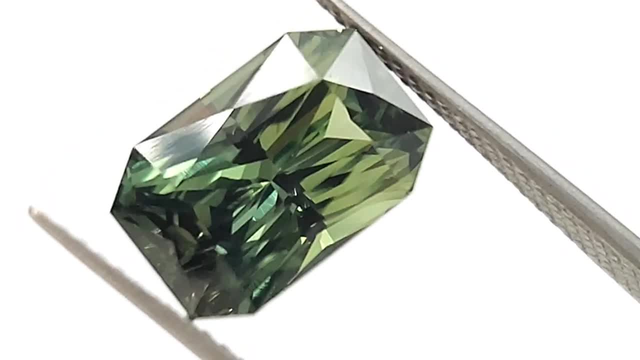 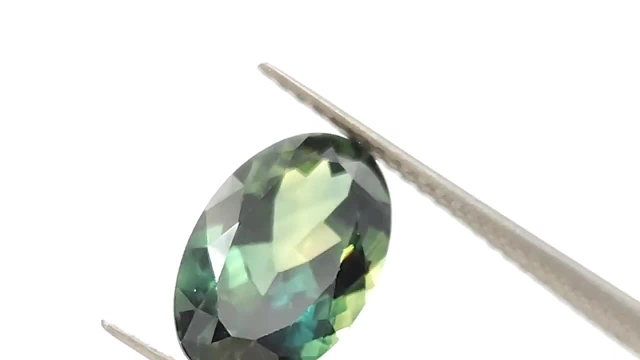 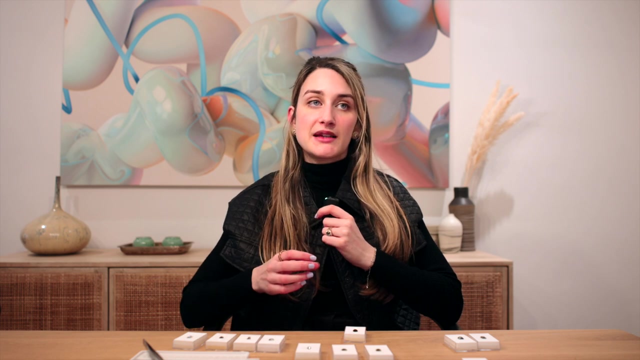 green- Okay, It's really green- in comparison to, like, let's say, this one that has highlights of blues, even a little bit of yellow green, all within the same stone, It's really eye-catching, And so that's why I would probably choose that Like. 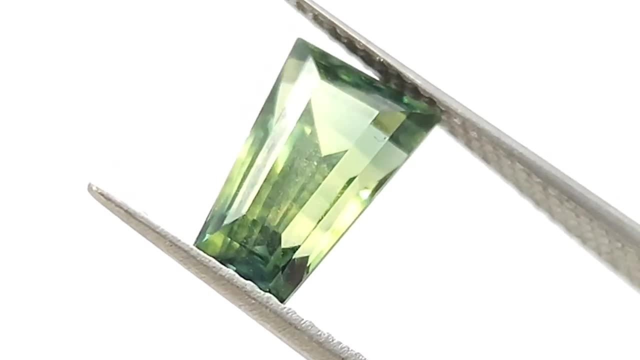 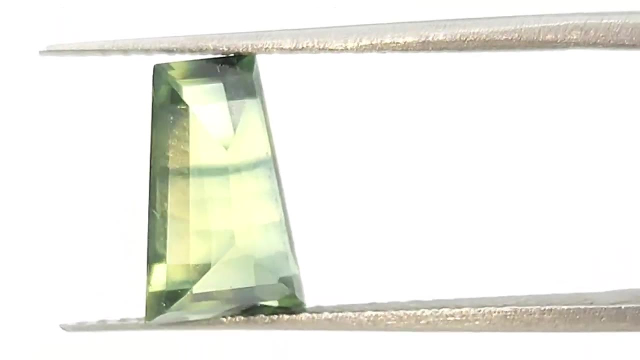 this one is the perfect example of color zoning. So this one is a lot more dramatic. As you can see, it's a very yellowy green in the middle and then you have blues on either end. So this is definitely an acquired taste, because you know it's not like the traditional aesthetic, but I 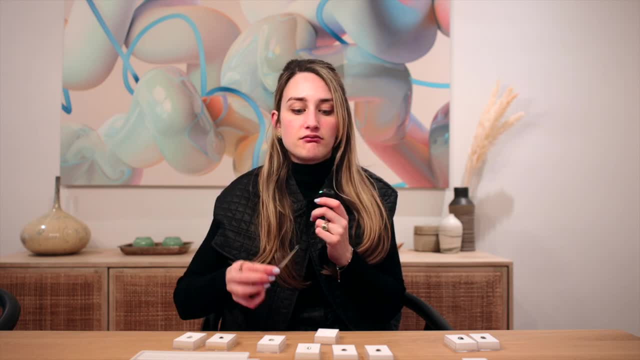 think there's a stone really for everybody, So I would definitely look for a stone that has highlights of blues in it, And that's why I love sapphire, because you can literally find anything and everything, So that's like an extreme example And otherwise they're going to really 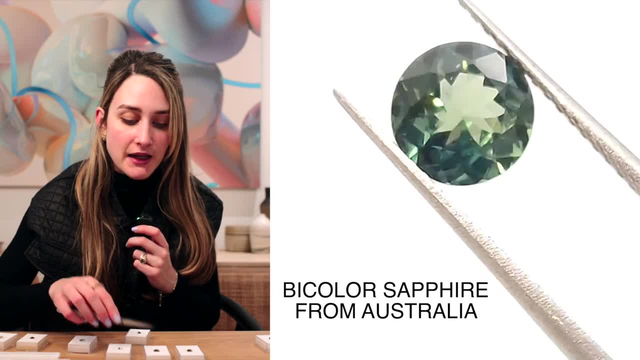 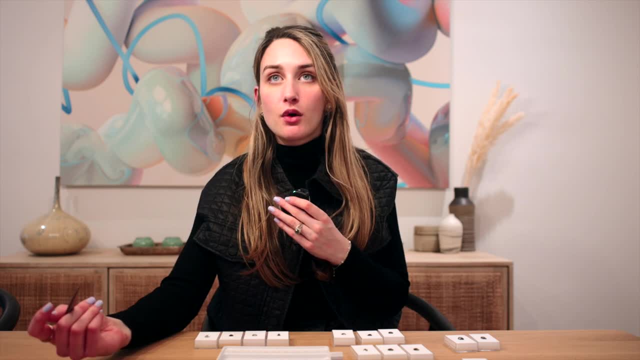 just be like mixed in and it just looks fantastic. All right, So now let's touch on prices. So most people generally want to start around the one carat mark, especially when you're talking about, you know, sapphire and green sapphires. you know it's not the price of a diamond. It's also not 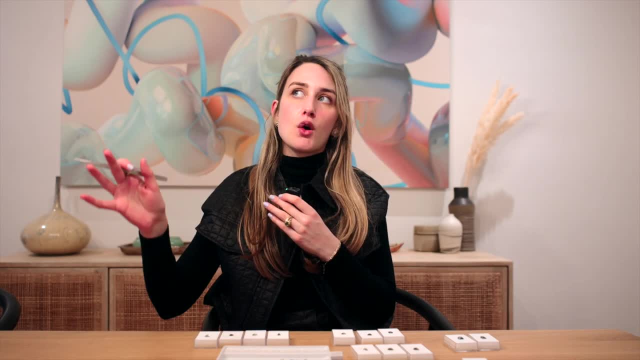 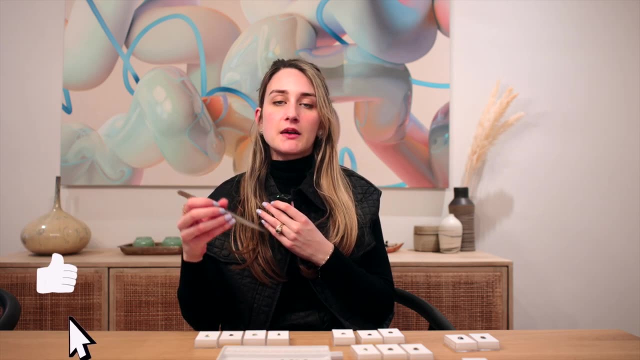 the price of a blue sapphire, right? So sapphires kind of go- I would say there's definitely a balance of popularity- that are going to influence the price, right? So a teal sapphire is going to be less desired than a blue sapphire, And so the price will be significantly less. So just to give: 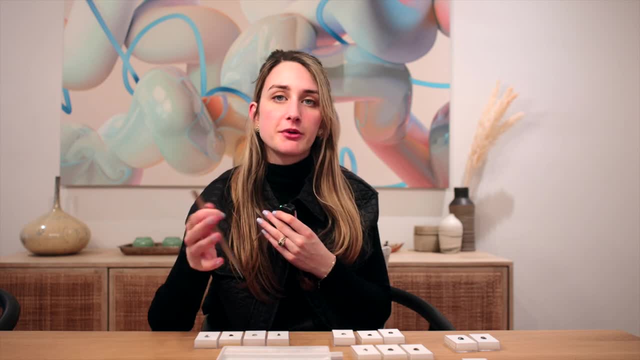 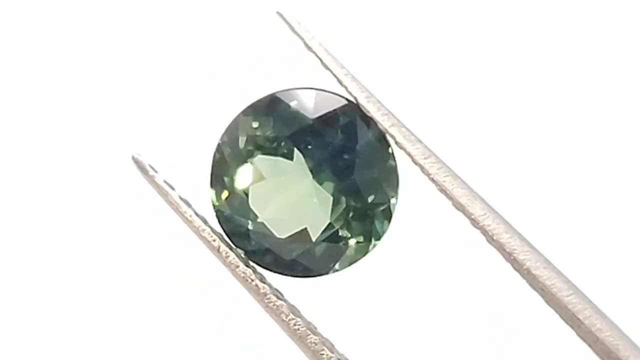 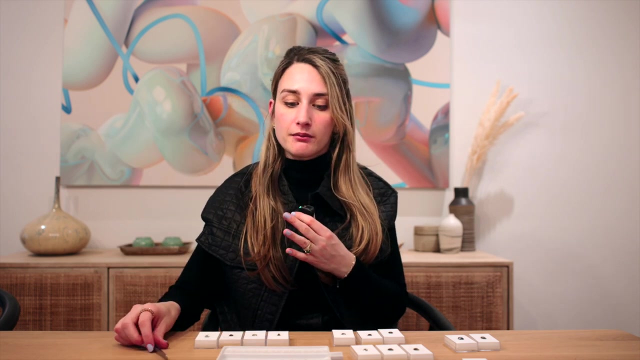 you a concrete example. let's start around the one carat mark, because that's generally what people start around. We have one carat, slightly greens to blues, and you're looking at about 1500 to, let's say, 2500 for a one carat stone. That's very, very good in terms of like engagement rings, I think. 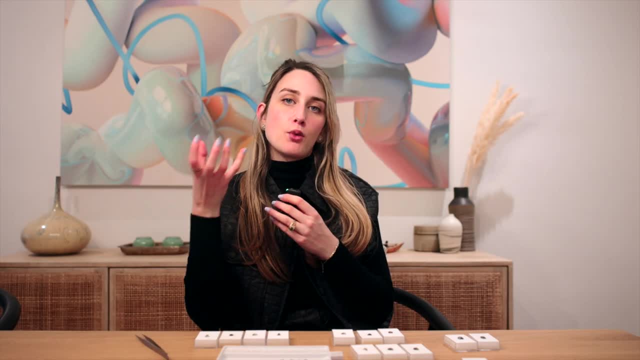 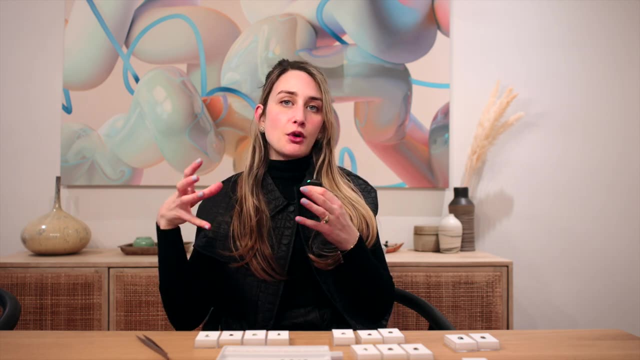 that the one thing that you want to keep in mind is that you're going to have a lot of people mind is that sapphires weigh more than diamond. Why is that relevant? It's relevant because if you have a one carat diamond, it's going to be about 6.5 millimeters in diameter, So the size of 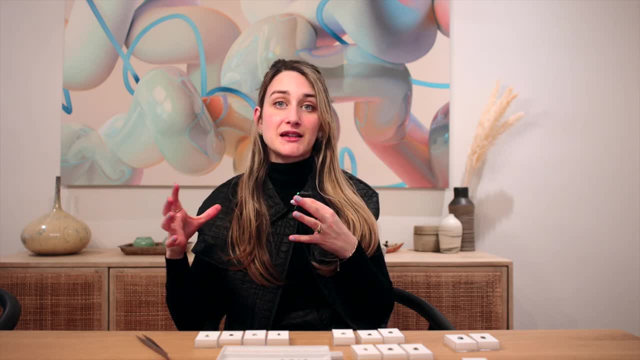 it versus a sapphire because it weighs more. a one carat is going to be smaller. It's going to be about six millimeters in diameter, So that's really important. You need to keep that in consequence, because you don't want to order a one carat and then you're going to look at it and 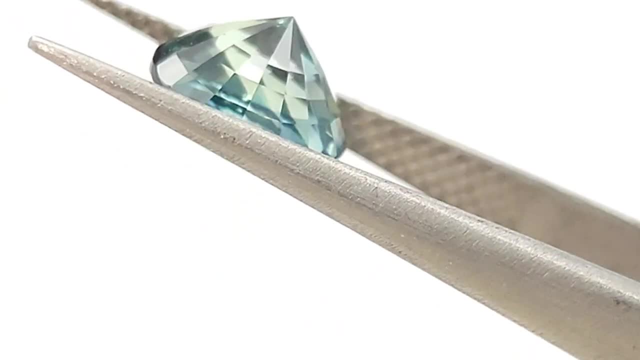 you're going to say, oh, it's a little bit small. Well, that's the reason why They also tend to be a little bit thicker on the bottom half, And so, again, it's not going to be cut like a diamond. 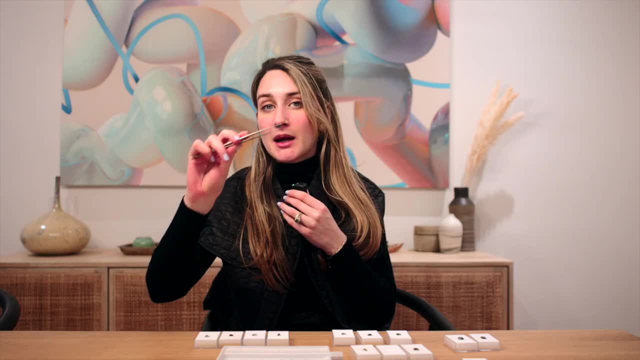 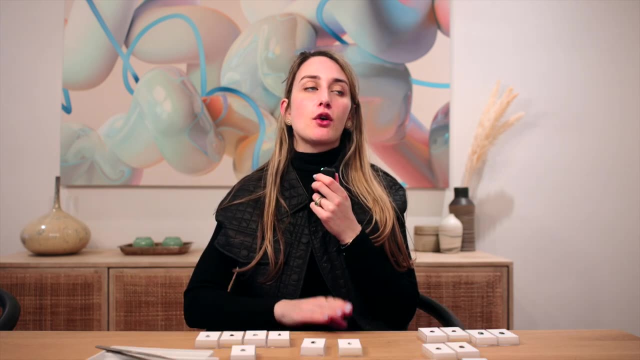 So even if you have the same cut as a diamond or the same carat away as a diamond, it can be a little bit smaller. So just keep that in mind. But generally the prices are pretty reasonable And I mentioned at the beginning of the video: you know if it goes too dark or too light. 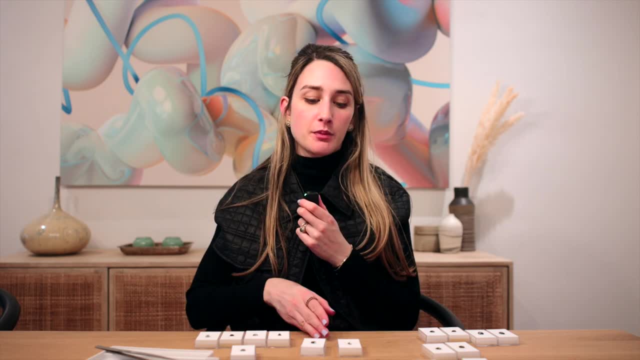 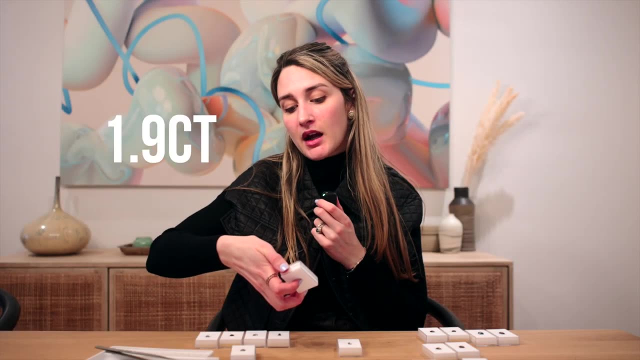 it's not good. It's definitely also going to change the price. So, for example, this one is a more desired green and you know you're looking at almost like 1.9 carats and you're looking at, let's say, 3,500.. 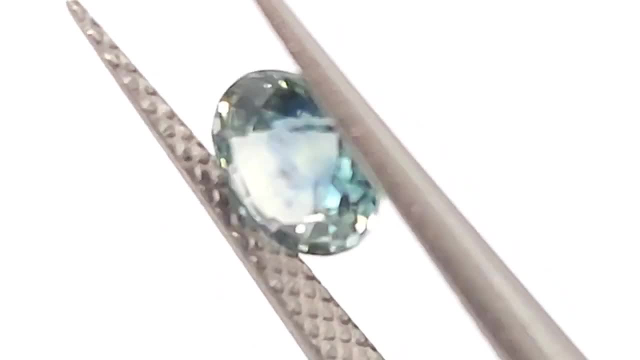 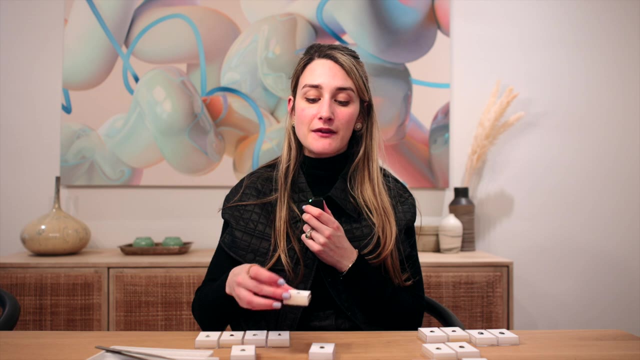 The stone versus this one is similar in size. However, it is a little bit paler and it's going for, let's say, 1,900.. So it's a very big price difference, even though it's just slightly paler. 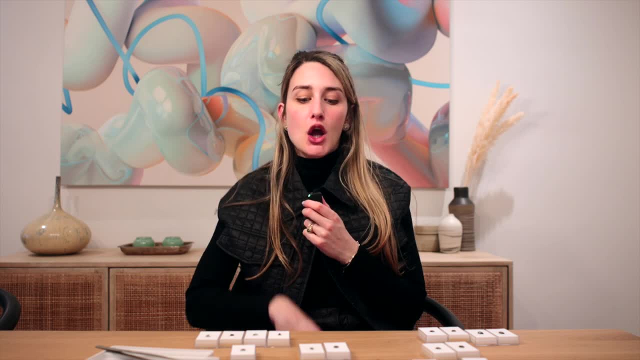 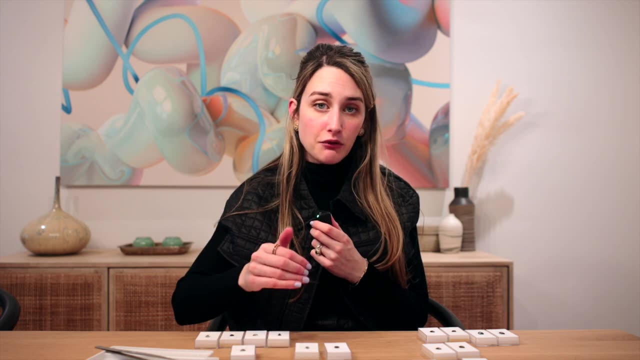 And so that's why sometimes clients, when you do have a little bit of a smaller budget going, a little bit paler is not the end of the world. It's also going to be a more vibrant stone because again more lights passing through. So it kind of is like a little bit of a personal 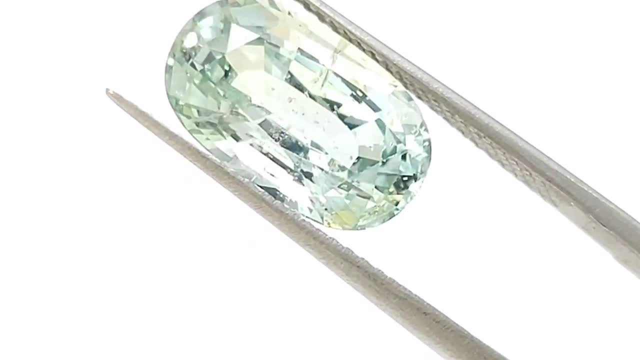 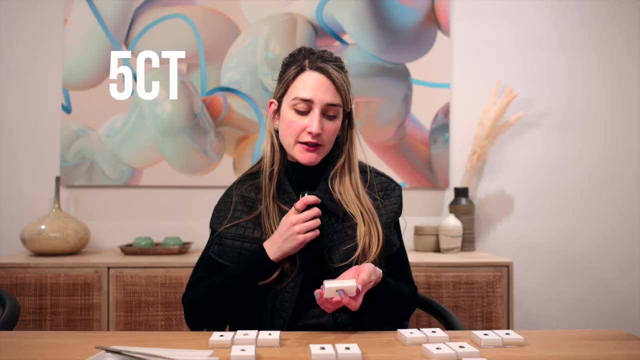 preference. I tend to like a little bit of a paler stone, Like this one, for example. it's very, very pale. I showed it earlier and you know you're looking at almost five carats and it's, you know, 4,300.. So the price per carat is: 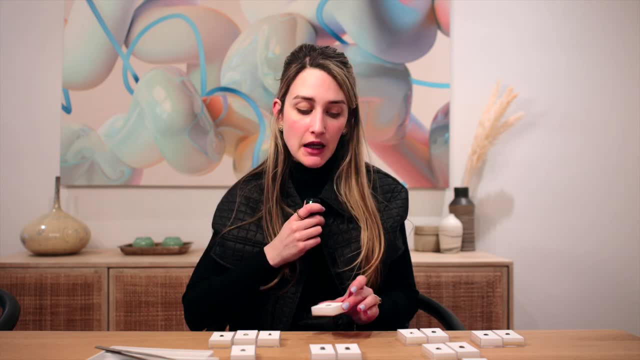 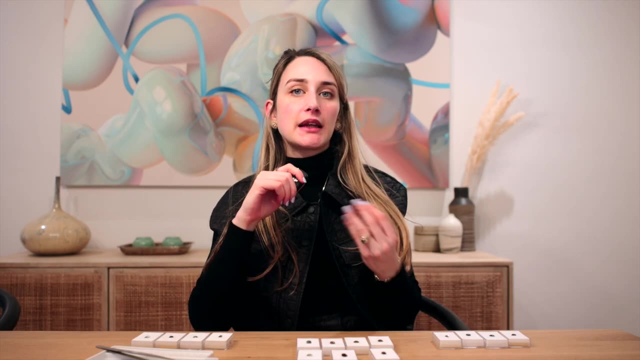 significantly less, like it's not even a thousand dollars a carat. So, as you can see, going too pale can really influence it. So now let's touch onto some eye candy, So let's go into the larger carat weights, just that you guys can get like a general feel for like the price. 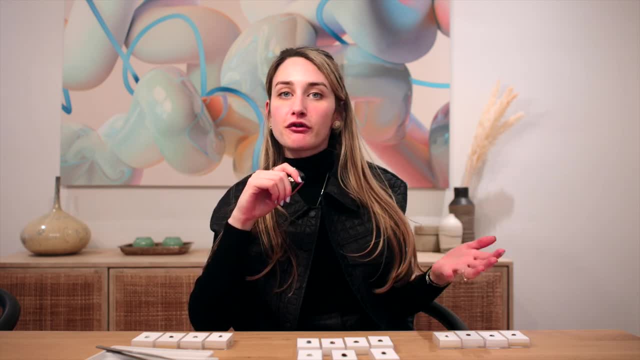 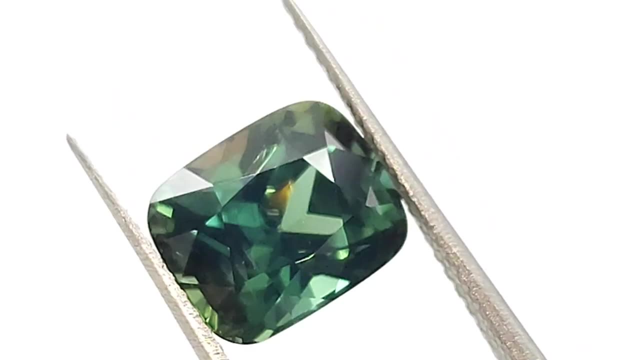 jumps. Usually, my clients are around the 2.5 to 3.5 carats, So these are more realistic if that's looking for. So this one is a beautiful cushion. It is a tiny bit dark, However, as you can see. it still has like a lot of light that passes through, So I don't mind it too much. but this bad boy is about four carats and it goes for like 8,000.. So it's about $2,000 a carat. I. 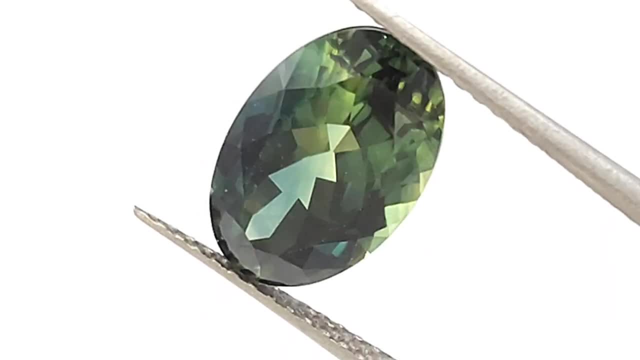 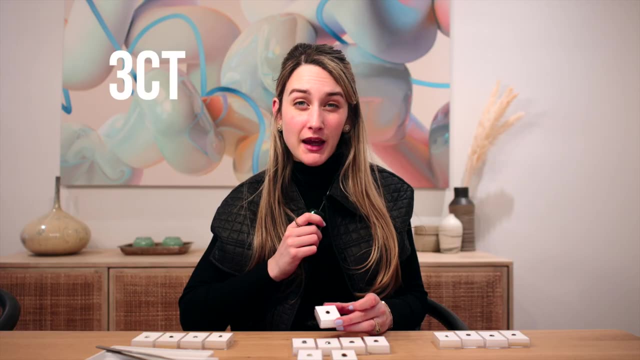 think that's very reasonable for the size. So this one's in the three carat range. I really love this one. As you can see, this is a slight light, lighter color zoning in the middle of the oval, which I really like. It's about three carats and it goes for 5,300.. So, yeah, this one's a. 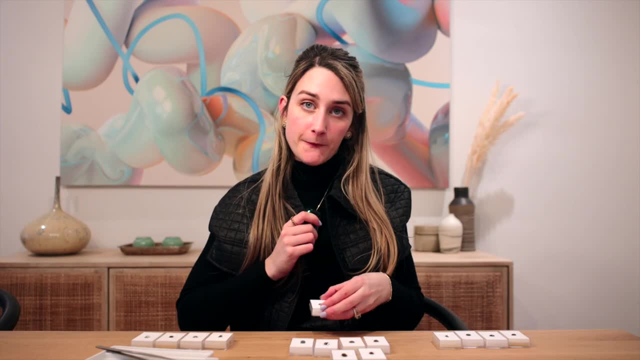 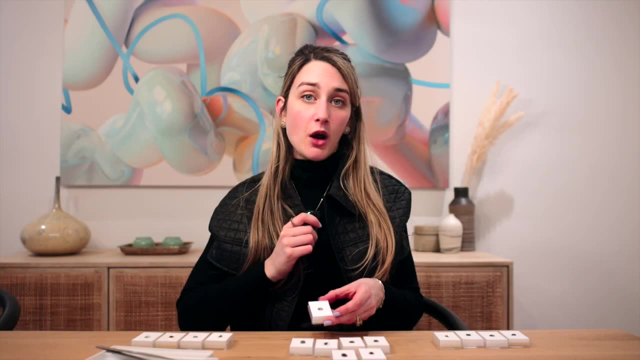 really one that I like. This one's a little bit more peculiar, This one, I would say, because it's a very specific yellow, like it's a yellowy green, and you don't see that many options like this. So this is a three carat but it goes for 9,000.. It has a really nice brilliance And, again, 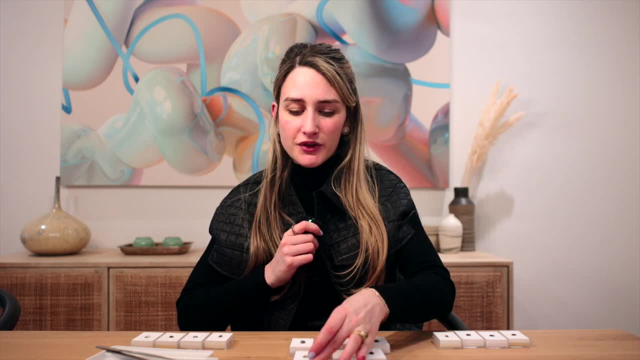 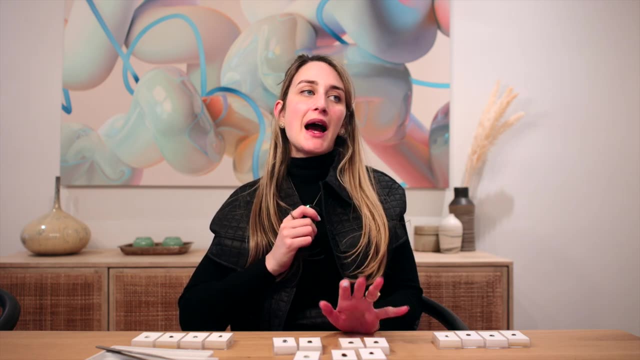 I think it's just because you don't really see this color, So it's it's hard to come by And I feel like that's why it's hitting a bit of a premium. So this one's a really interesting comparison. So I get a lot of clients who will ask me for no heat stones. 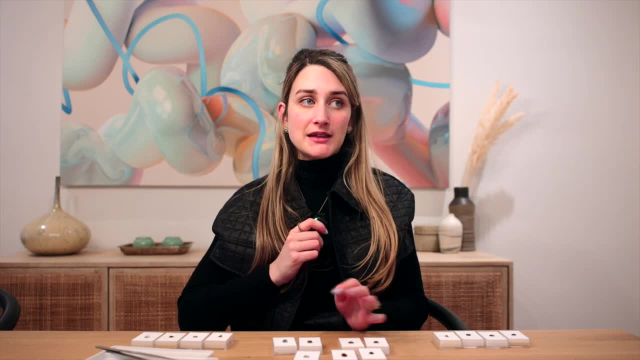 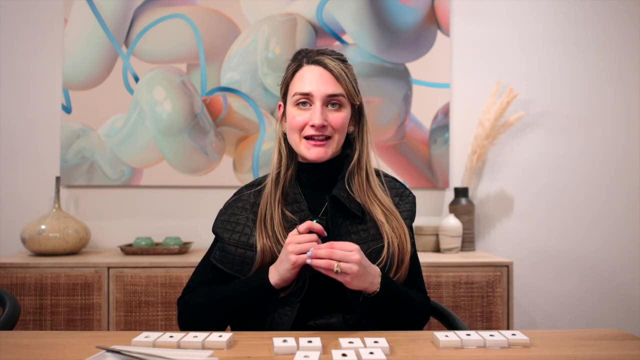 I want to really specify that having a heated stone is not bad right. It's just a tiny enhancement that still considers your stone natural. It's just that when you have one that isn't heated, if you're able to find one that isn't heated, it means that it's naturally occurring. 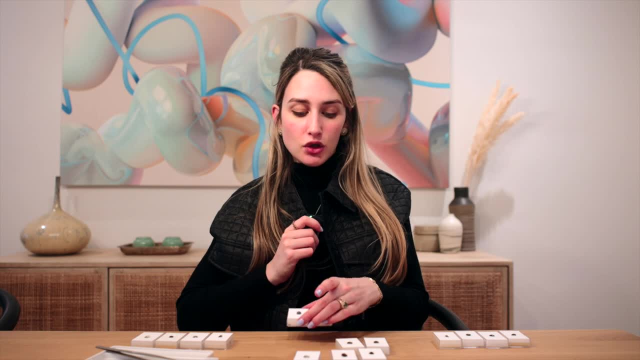 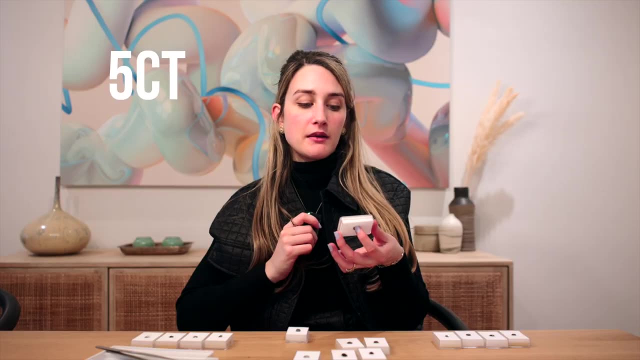 like that, which drives the price up quite significantly. So these are two examples of teal sapphires. So this one is a little bit green and it goes to five carat for about $9,000 versus. this one is a no heat, As you can see. 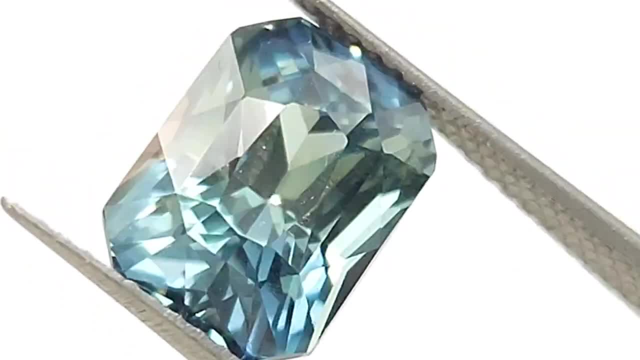 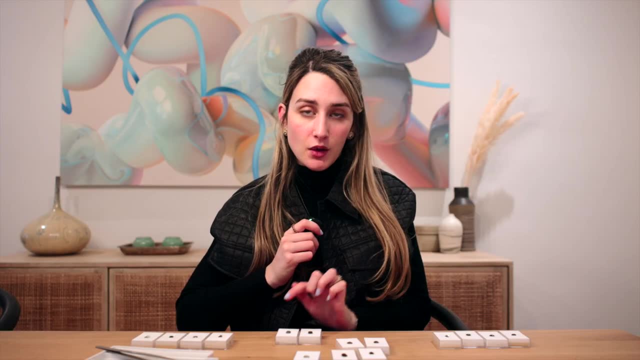 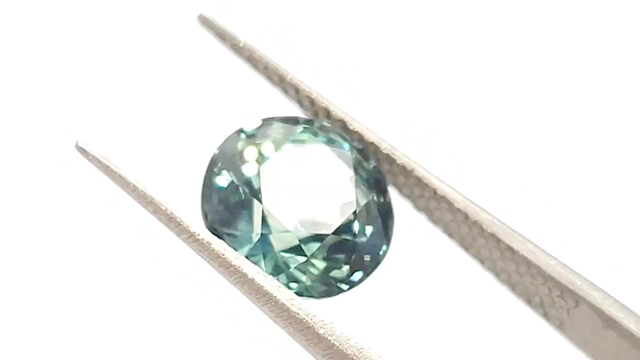 it's a little bit more blue and about the same carat weight, And you're going for 20, 20,000 over $20,000.. So the price jump is quite significant. Had it not been heated, obviously, it would have been a lot less. just to give you an idea, See, we also have this one here. 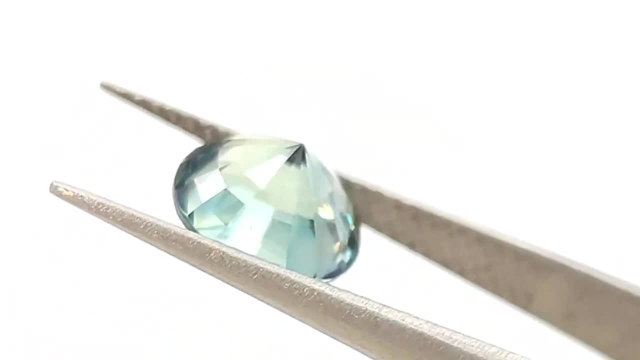 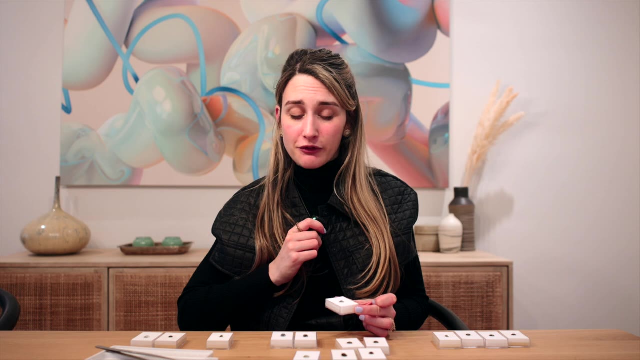 That's a no heat for about 2.58 carats and it's over 7,000.. So had it not been heated- because, as you can see, it's a lot paler- it would have been significantly less, probably in the three to.